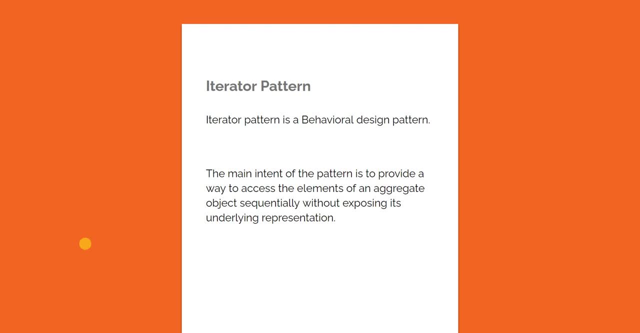 to access the elements of an aggregate object sequentially without exposing its underlying representation. So what this means basically, is that this design pattern was built so that we can segregate the implementation of a collection from its iteration. That is what is the underlying intent of this particular design pattern. So if you think about solid design, 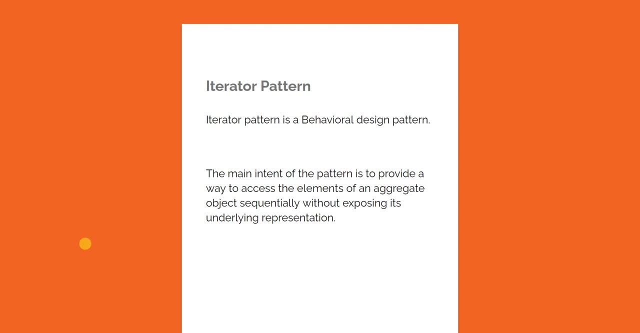 principle. also, it makes a lot of sense Because the collection, which is an aggregate of object, should not have the responsibility of how to iterate through the collection. That responsibility should remain with the iterator itself, and that's what this design pattern tells us. So let's go through. 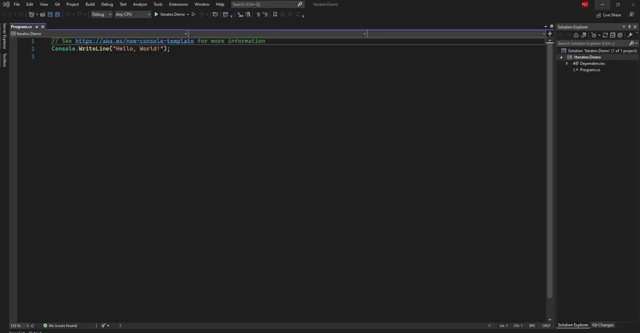 an implementation, and it will become much more clearer when we go through individual code. So, for this purpose of this implementation, we'll have two things: We'll have an aggregate, which is nothing but a class which will hold a collection, and then we are going to have 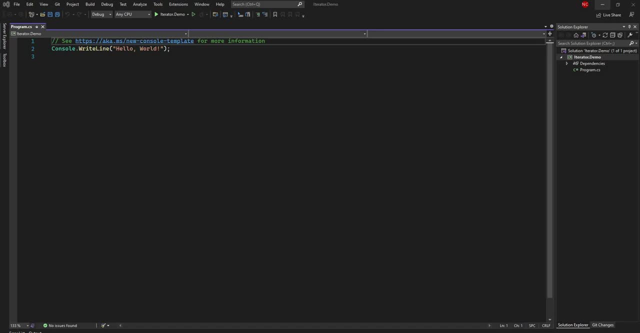 an iterator. Iterator is nothing but a class which will be responsible for iterating through the aggregate or collection. So first let's start with aggregate, Though aggregate and iterator are related, so we need to create both of them almost in parallel. but let's start with aggregate first. 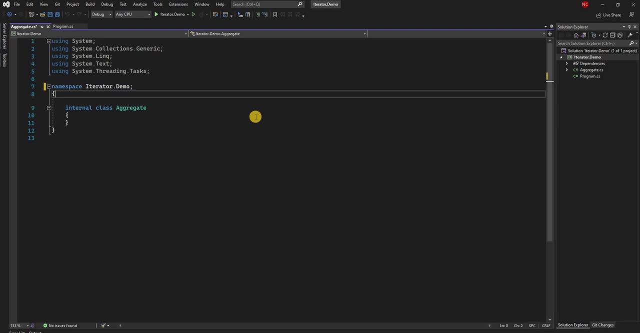 So for the aggregate class, let's change the implementation a little bit to use the NET 6 methodologies. Okay, now for the aggregate class. first of all, we are going to make it as generic, so that we can use the same aggregate class for different types. 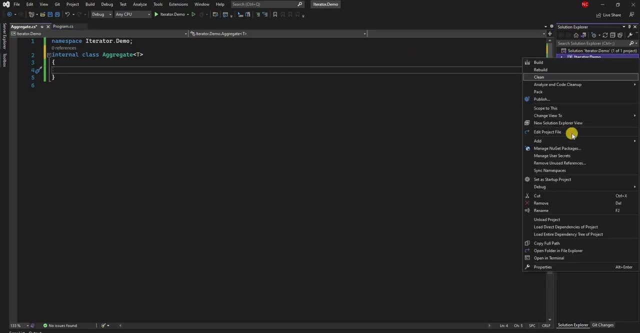 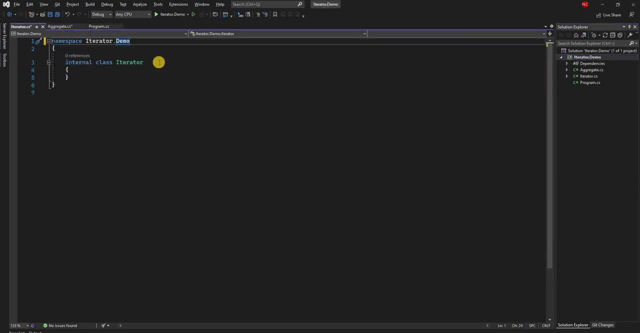 and then the aggregate needs the iterator. So let's create the iterator class. And since iterator will also have generic, but since you know that we will be dealing with interface and not the concrete class, so for iterator also, I'm going to create an interface. 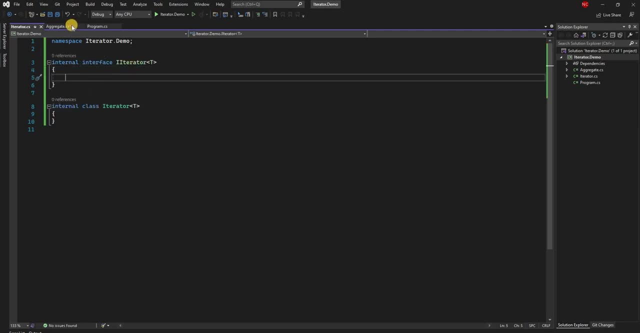 For the time being I'm not going to give any message. We'll come to the method later. It will become clear what all method we need in iteration once we go to the aggregate. So let's go back to the aggregate and now for aggregate, what we 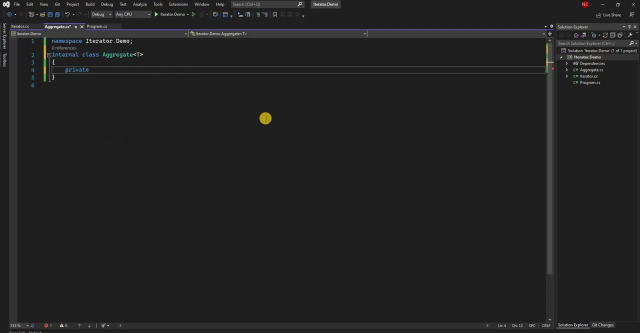 are going to have is we're going to have a private iterator of t and then we are going to have a private list of t which will hold the actual value, and this one can be new list of t And this one can be new list of t. 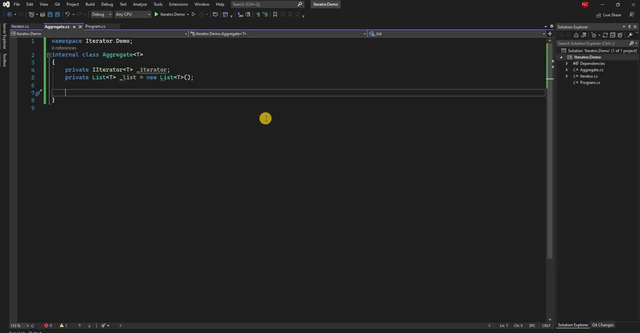 So once we have that, now we would need some way to expose the value, because the iterator would need the values to iterate through, and also we would need a way to add values So we can support both through a single method, So we can have public. 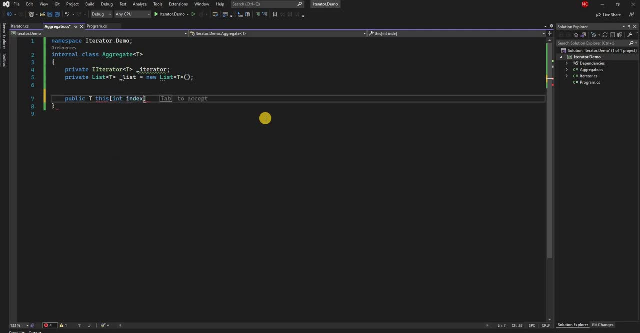 these so we can use an indexer index, and then this does some job for us. so let's make it a little bit more clearer. So we have a get which will return the value from the list based on the index, and then we'll also have a set, and for the set, what we're going to do is we're going to have 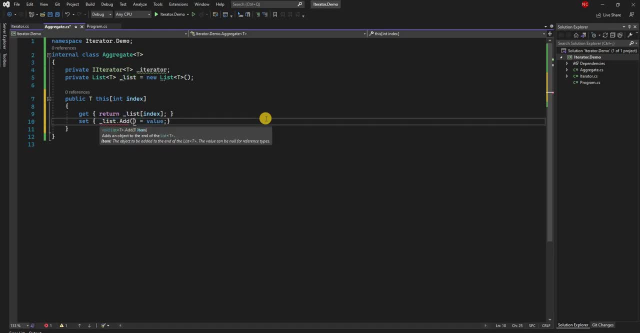 listadd, and then we're going to add the value to the list. So that's our indexer, and then what we are going to do is we are going to expose the iterator. for that we can create public iterator of t iterator, and for that what we can have is we can have a little bit. 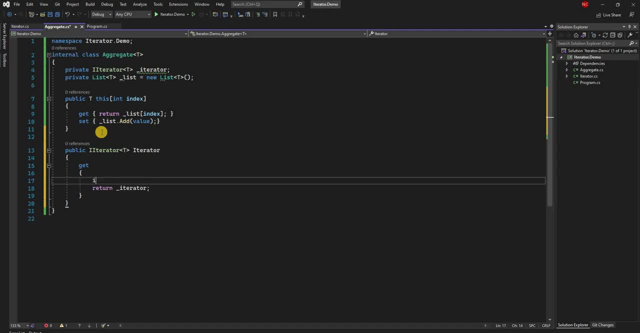 we cannot just directly return the iterator. we have to do: if iterator is equal to null, then say iterator is equal to new of iterator of t and this is going to be the concrete class: iterator of t, but iterator of t if we go back to the iterator, since right now the iterator does. 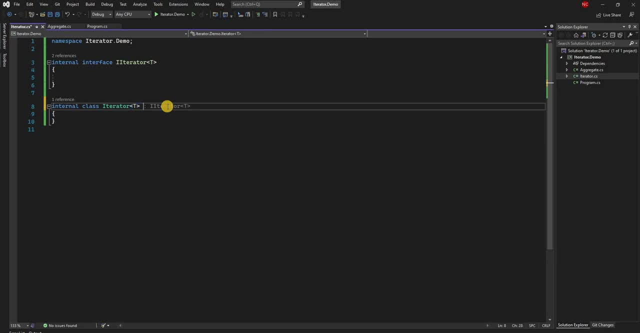 not implement iterator. that's why it's destroying this error. but I'm going to just implement iterator and we should be good. So we started with iterator. we return the iterator. now the aggregate is just holding the object and iterator will be responsible for iterating through the object. The other thing we would need for iteration is the count. 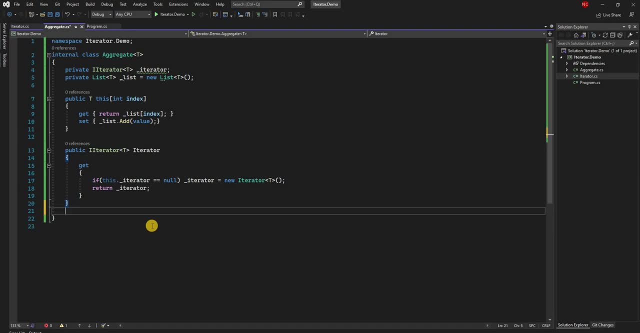 Basically what is the total number of item the aggregate contains. So for that we'll have a count method and for the count method we can just have underscore, list, dot count as the value. Now let's extract an interface and let's keep the interface in current file itself. 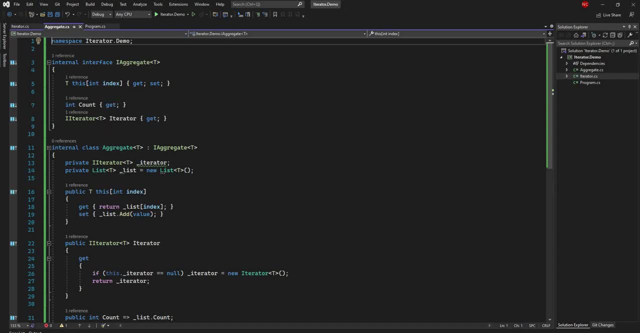 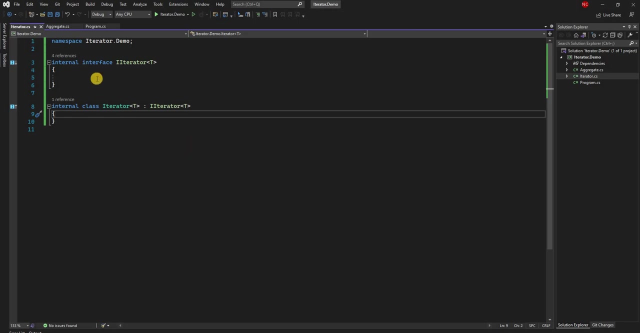 So we got our i aggregate, which has these three particular methods: One is the index, one is the count and then finally returning the iterator. So our aggregate is ready. Now let's go back to iterator and let's try to finish it. Now for the iterator, the first thing. 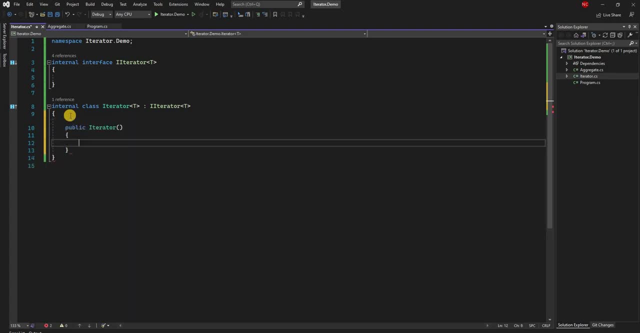 we'll need is the aggregate. So in the constructor of the iterator we are going to have i aggregate of t and aggregate, and let's declare this privately and also just for consistency, given that here all the name starts with underscore, Let's keep underscore name here as well. 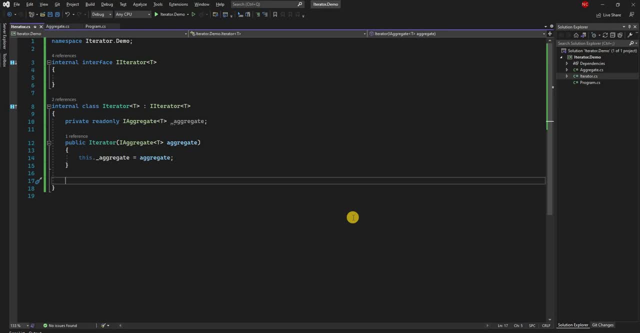 Next, what we are going to have is for iteration. what are the things we need? First thing we need is a current value. Second thing we need is: is there any item left? Third thing we would need is a way to move to the next object. 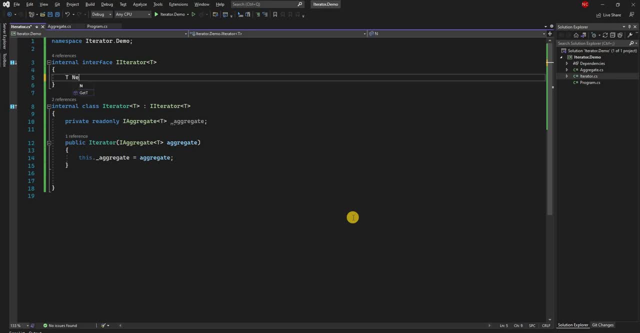 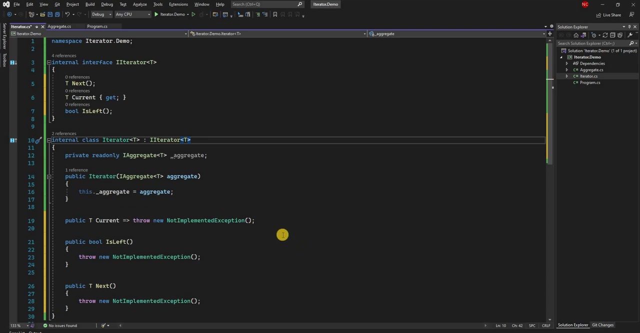 So for that we're going to declare t things. First thing we'll say is the next method. Next, the second thing is the current, which can be just a get, and the last one is: pull is left. So we'll have these three. So let's go and implement these three. 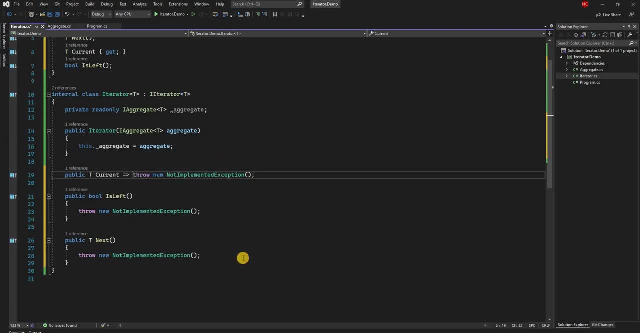 So for the current it is going to be nothing but aggregate of index. So we need an index. So let's declare this. So we are going to declare an index here and the index will of course start with zero. That's the first one. 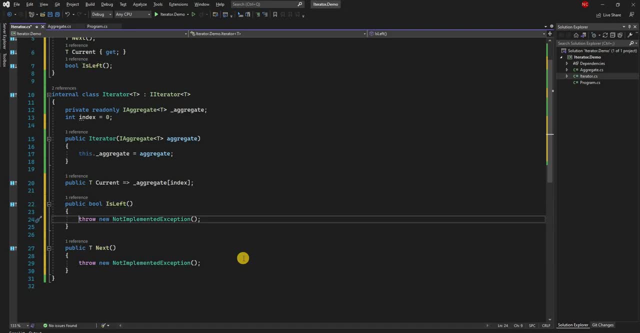 Next thing let's try to implement is left. So what is the logic of is left Is left is. so let's say we have two items, zero and one, and the count is two. Till we are in index of one, the item is still left. But when we go to index of two, there is no item left. 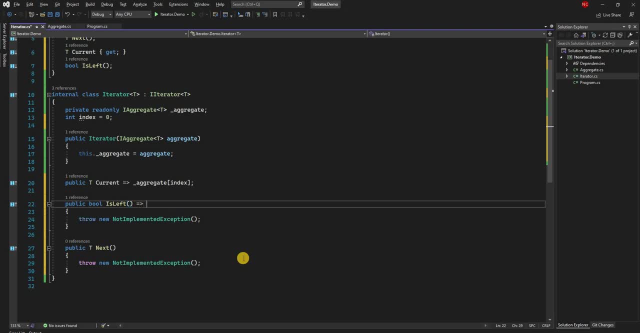 than the count. So for that what we can do is we can just implement it inline and we can say: index is less than aggregate underscore, aggregate dot count. So that will be the implementation of isLeft and then, finally, we go to the next. So whenever we are doing a next, so we are in zero, we are asking for next First. 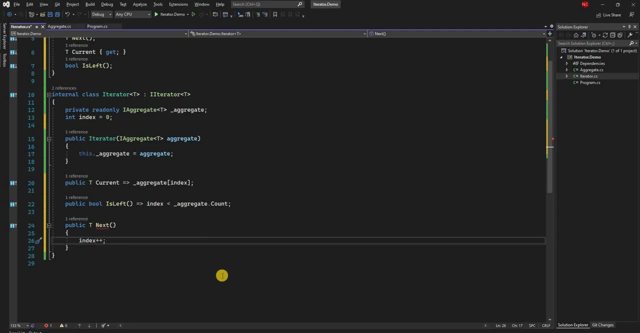 thing. what we are going to do is we're going to do index plus plus, so we'll increment it, and then we are going to do return, and here the autosuggest just gave it aggregate of index, which is correct. but there will be a condition. We'll check: isLeft then, yes, aggregate of index. If nothing is left, then we are. 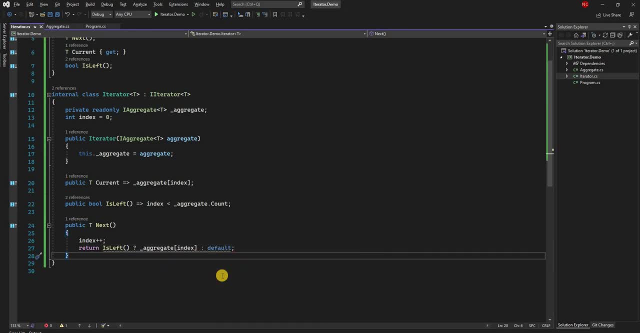 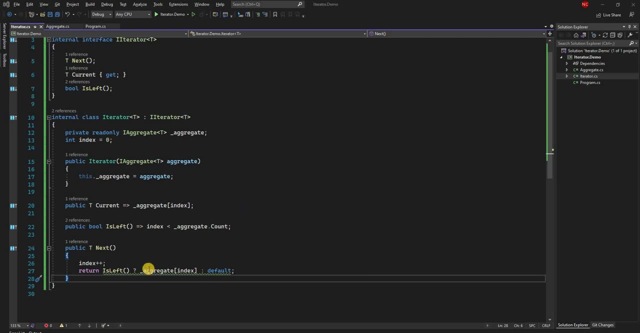 just going to return the default, which is null. So now we'll go back to program. Well, before we go back to program, we have to define the object which we have not defined. So what we are going to do is we are going to define the object which we have not defined. So what we are 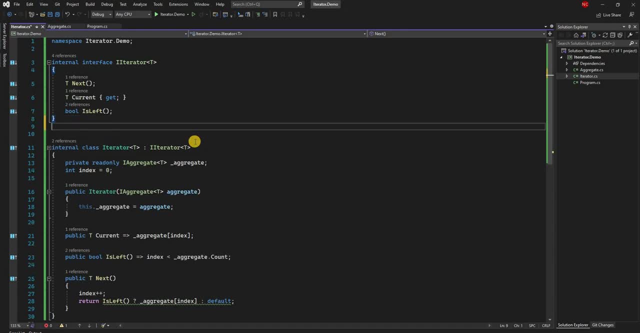 going to do is we are going to define the object which we have not defined. So what we are going to do is we are going to deal with. so let's say we are going to deal with a person type. Let's just create a record type here so we can say: 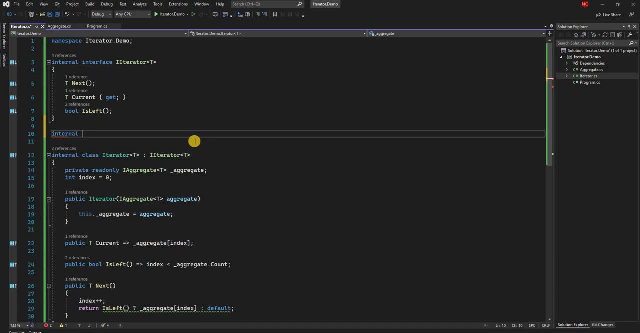 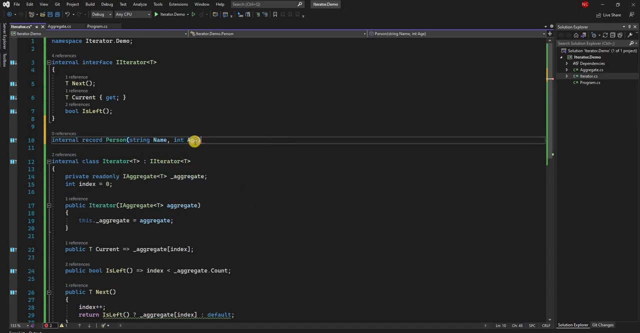 internal internal record person and for simplicity let's say person have to name and then int age. These are only two things for the time being. So we declared our record type which we can use with iterator and aggregator. We can use multiple object. given that these are generic, these two classes can be used. 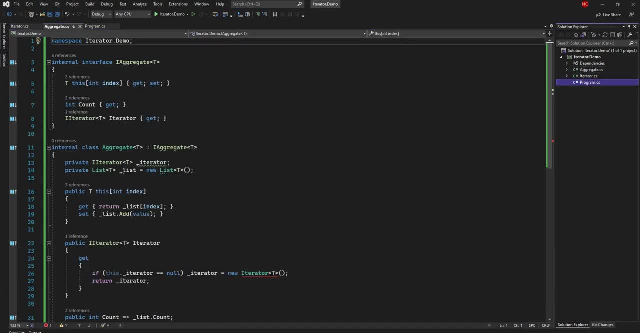 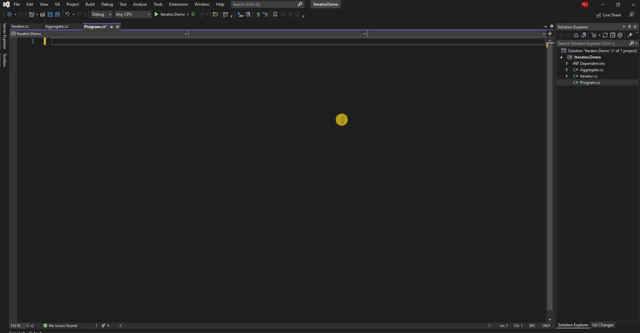 for iterating through any object, for that matter. This is the iterator pattern we implemented. Now let's go and see the code in action. So, first thing, what we are going to do is var persons is equal to new aggregate of person. Now we have to add the 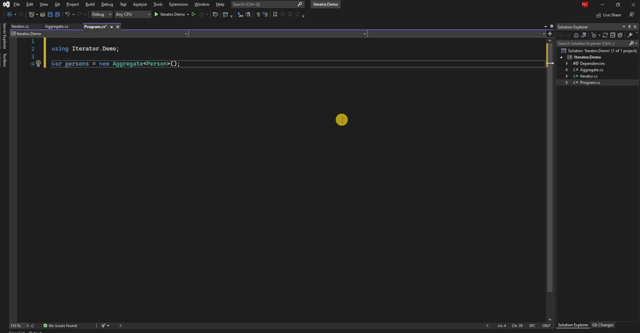 namespace. Okay, so now we have the person object. Let's go and add few person here, So I can say a persons of 0 is equal to new person, and here for the name we can say John, age 30. and then let's copy it couple of times and add two values. So first one, let's say it's Jane, age is 20.. 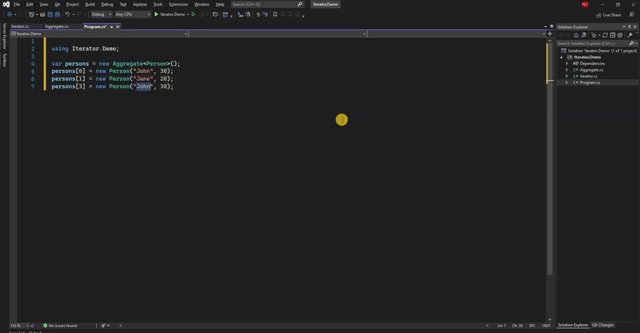 And then three: name is Michael and age is 10.. Now let's get the iterator from it So you can say: var iterator is equal to persons, dot iterator, Iterator is a property. and then what we can do is we can have a simple while. 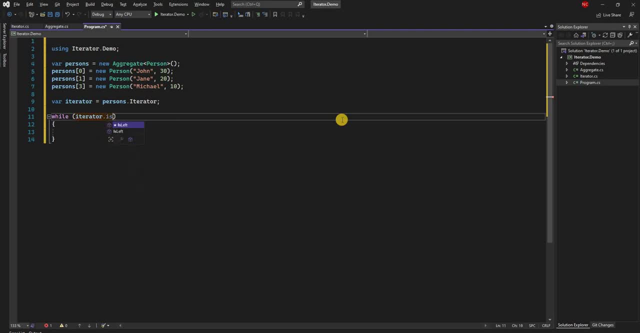 condition. and here we can say: iterator dot is left. If left, then we're going to have console dot right line. and here we can say: iterator dot current. You can print the current and then we'll just move next. That's all. So now. 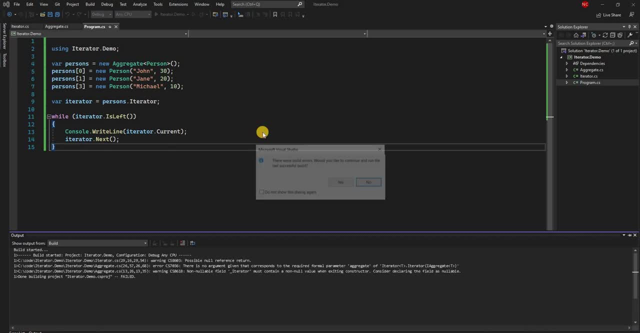 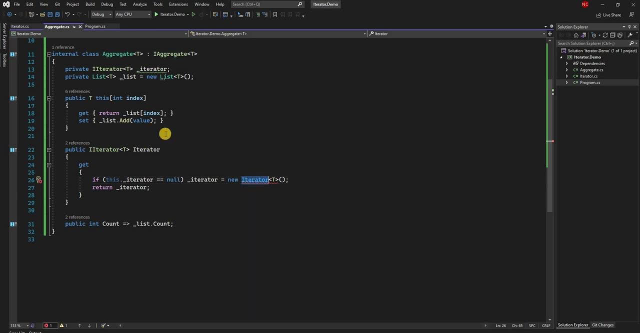 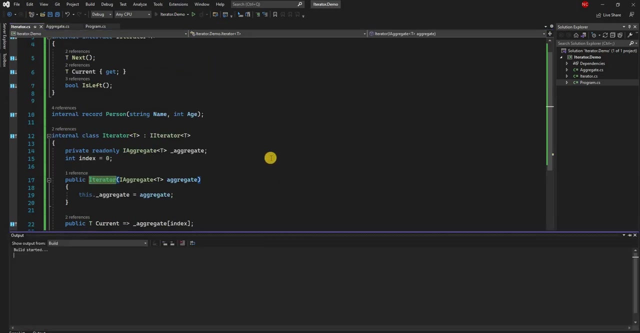 if we run this application, it should print John, Jane and Michael. We have an error We have to pass. remember we updated the iterator to take the aggregate in the constructor, which it has to, and for the aggregate it is not nothing but this. So now let's run the program and if we run it, we should see. 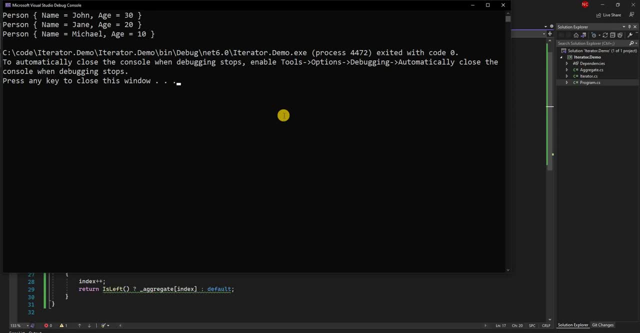 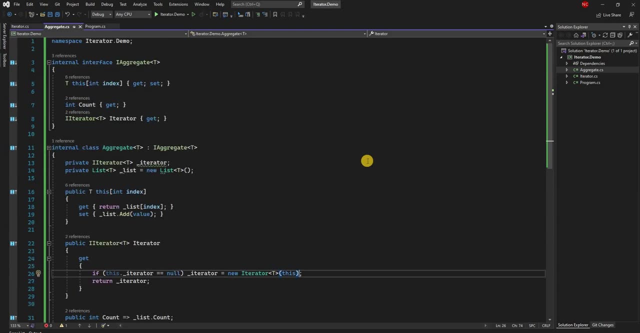 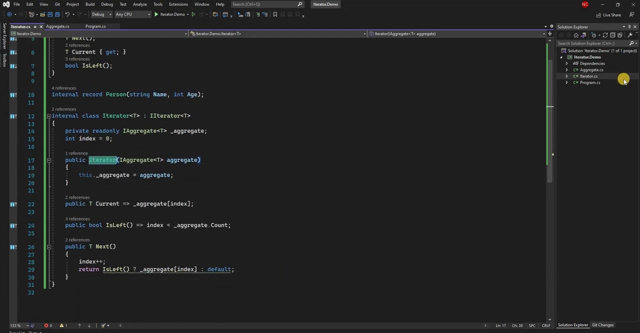 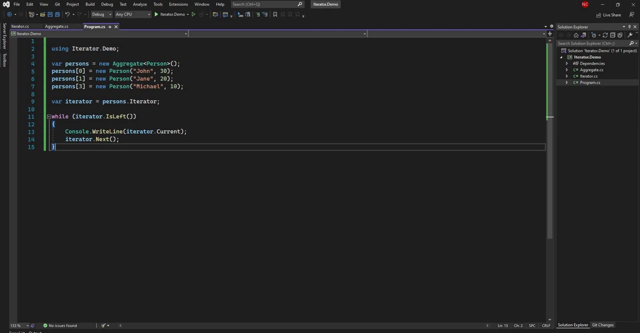 John, Jane and Michael, as expected. So this is in a nutshell what iterator pattern is and, as you can see, it's very simple to implement, of extremely generic implementation of iterator pattern which can be used with multiple object, But in dotnet C sharp, given, we already have something called I enumerator. 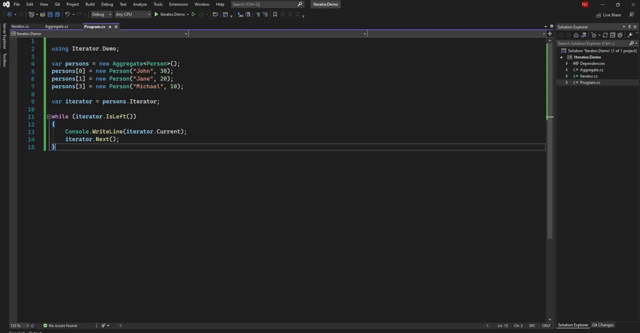 which is an implementation of iterator design pattern with little bit of difference, meaning it is little bit sophisticated, in a sense that when you do for each loop itself, it walks through the iterator, gets the next item and gives you that value. So you really don't need to implement this kind of 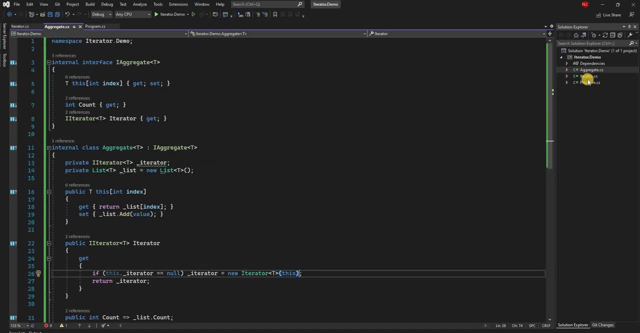 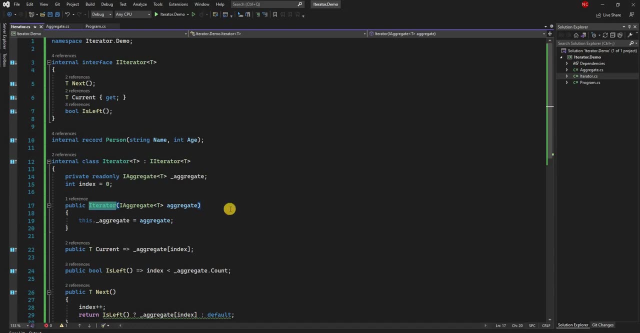 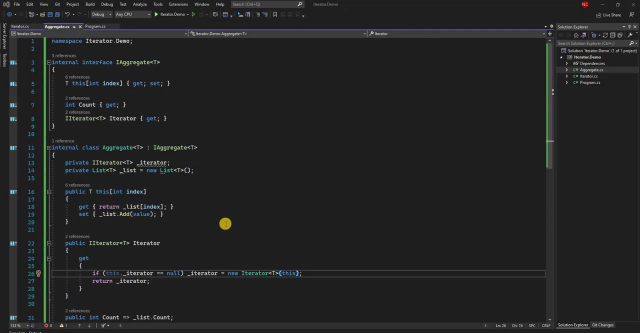 implementation, but this is the high-level implementation of iterator pattern. There are situation where you might have to create your own iterator, in which case it will be useful. Otherwise, you can just go ahead with I enumerator, and it should work for you. But I enumerator can be used only with I enumerable. So that's all I wanted to. 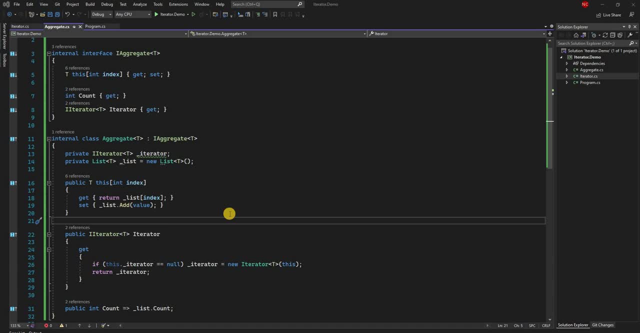 cover for today's video. If you like this video, please give me a thumbs up, and if you are new to my channel and you think you are getting value out of my channel, please subscribe to my channel and thanks so much for watching this video. 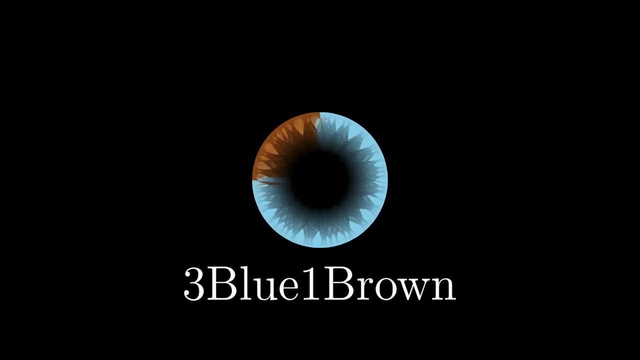 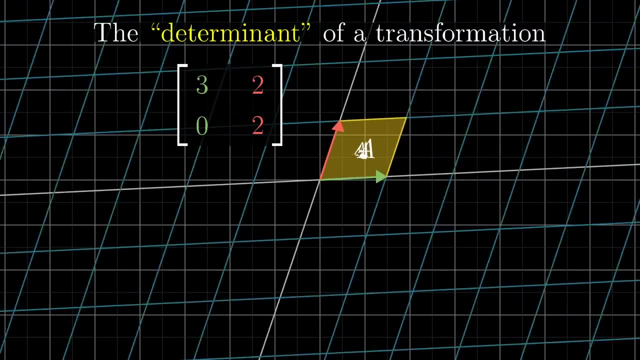 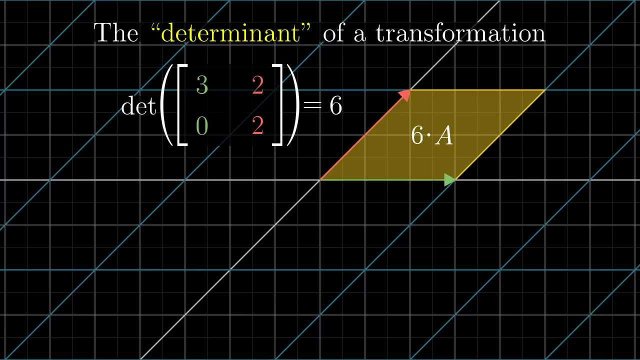 Math is sometimes a real tease. It seduces us with the beauty of reasoning geometrically in two and three dimensions, where there's this really nice back and forth between pairs or triplets of numbers and spatial stuff that our visual cortex is good at processing. For. 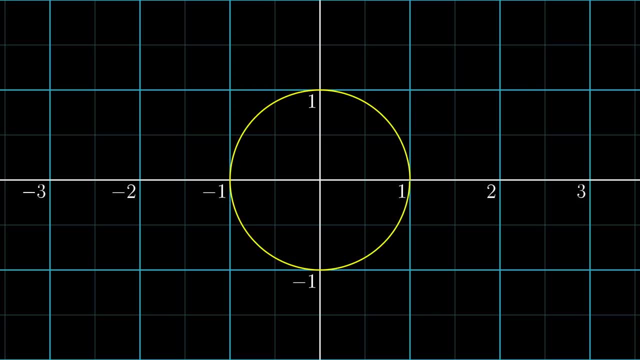 example, if you think about a circle with radius 1 centered at the origin, you are in effect conceptualizing every possible pair of numbers- x and y- that satisfy a certain numerical property: that x2 plus y2 is 1.. And the usefulness here is that a lot of facts. 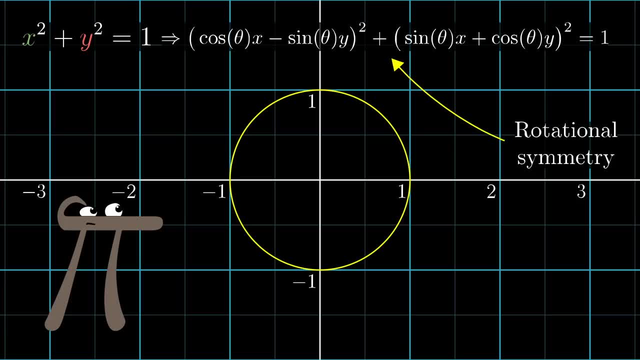 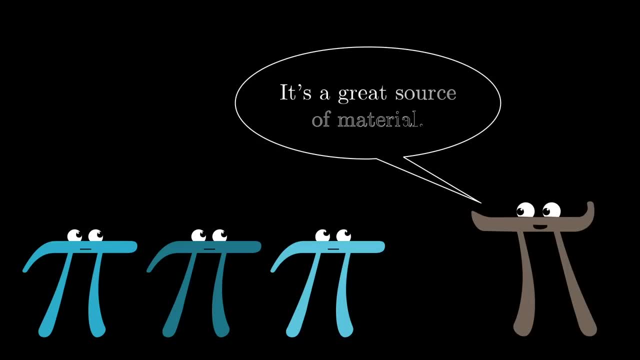 that look opaque in a purely analytic context become quite clear geometrically, and vice versa. Honestly, this channel has been the direct beneficiary of this back and forth, since it offers such a rich library of that special category of cleverness that involves connecting two and three dimensions of a circle. 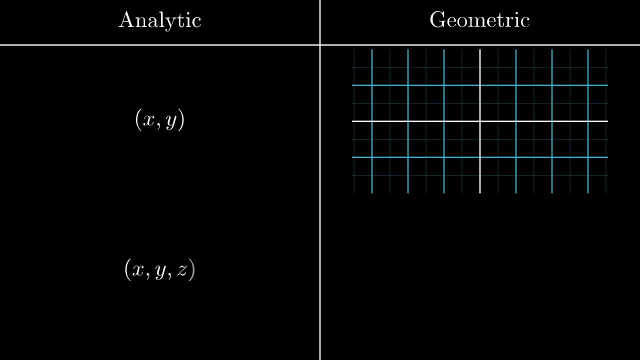 And I don't just mean the general back and forth between pairs or triplets of numbers and spatial reasoning. I mean this specific one between sums of squares and circles and spheres. It's at the heart of the video I made showing how pi is connected to number. 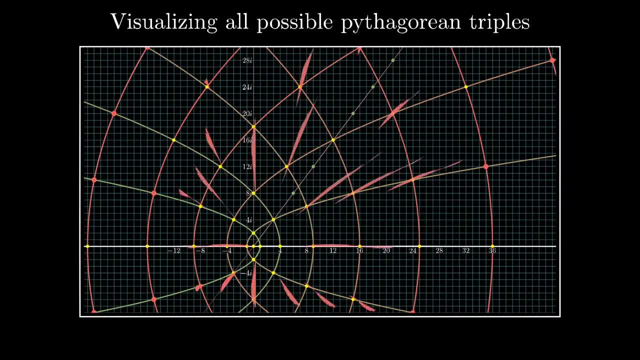 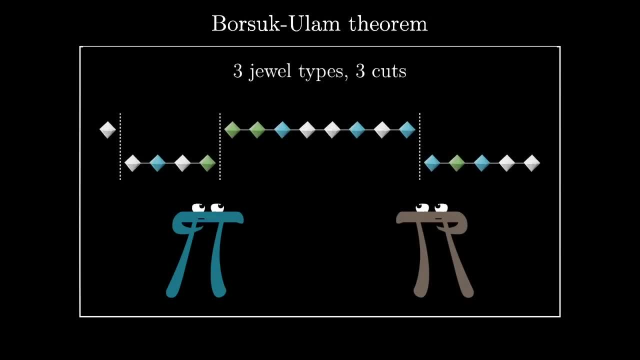 theory and primes, and the one showing how to visualize all possible Pythagorean triples. It also underlies the video on the Borsuk-Ulam theorem being used to solve what was basically a counting puzzle by using topological facts. There is no doubt that the ability to frame analytic facts geometrically is very useful.